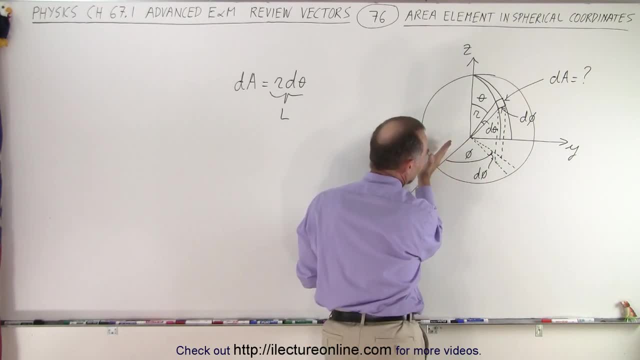 Notice, the angle from the x-axis to the first line is phi, And then the angle from the x-axis to the next line is phi plus d phi. That's a change in phi d phi, So that length there would be called r times d phi. 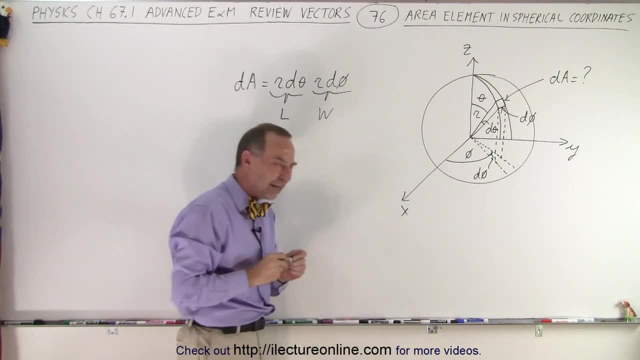 And that would be, let's call it, the width of the rectangle. But that's not the whole story. This is where it gets a little bit strange. It turns out that's only the case in a very specific situation, That's if the area element dA is along the xy plane. 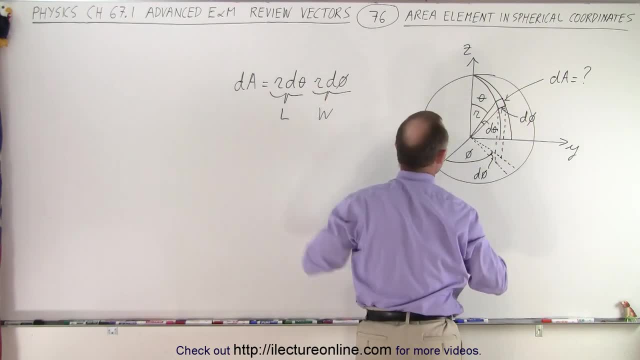 That's when the area element here is exactly equal to that, But that's only the case on the xy plane. Why is it not the case? Well, simply take a look at it. So, if you see the two lines that go from the equator of the sphere to the pole of the sphere, 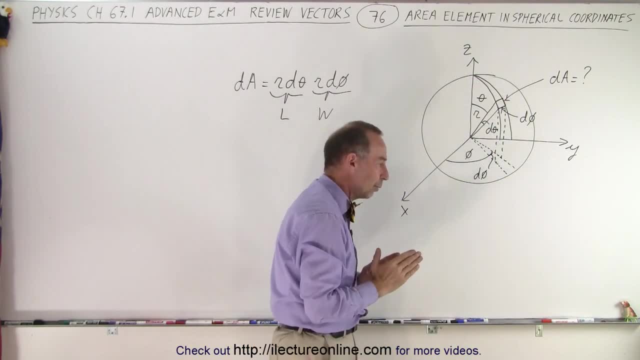 just like on the Earth, the longitude lines that run parallel to each other. well, actually, they don't run parallel to each other, because when we get to the equator, we run parallel to each other. When we get to the pole, they converge together at a single point. 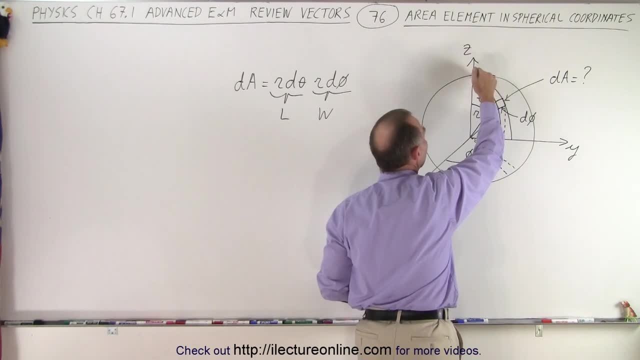 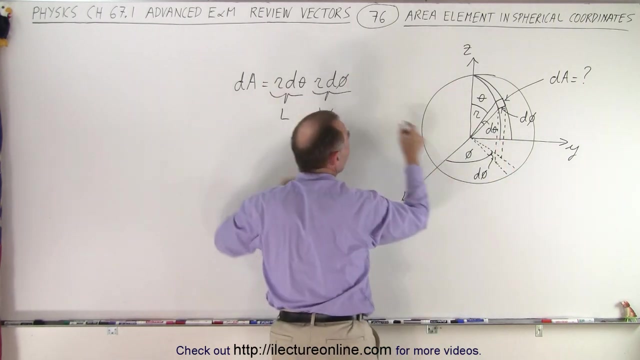 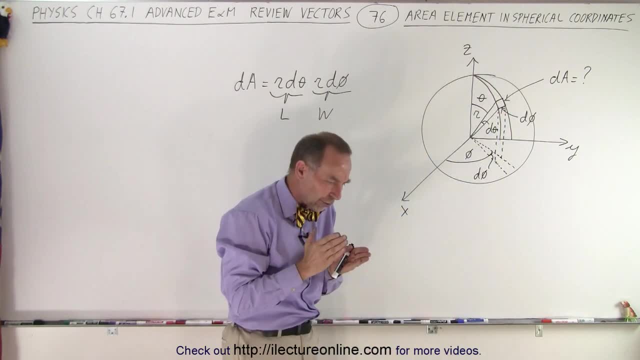 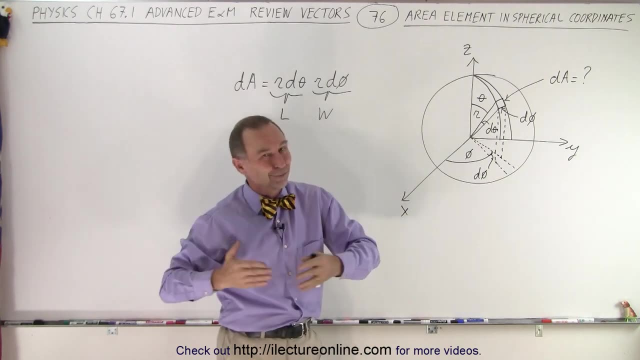 and that, theta being zero degrees, it's equal to zero. So we're looking for a trigonometric function where, when the angle is zero, it's zero, and when the angle is 90 degrees, it's maximum. Well, that's the sine of the angle. 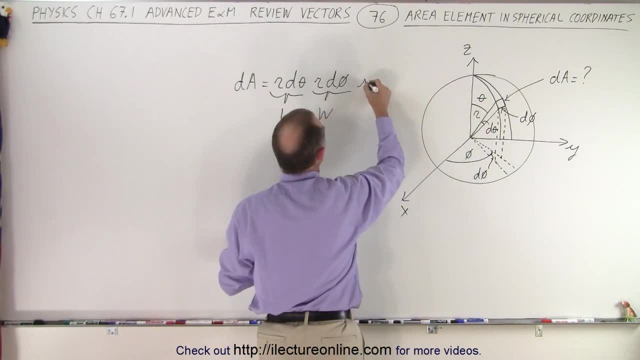 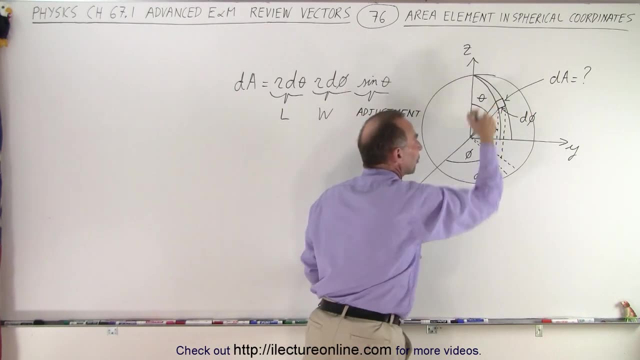 In this case, the angle is theta, So we also have to multiply that times the sine of theta, and this is the adjustment that we need to make in order to compensate for, essentially, the geodesic right, the lines that would normally run parallel to each other. 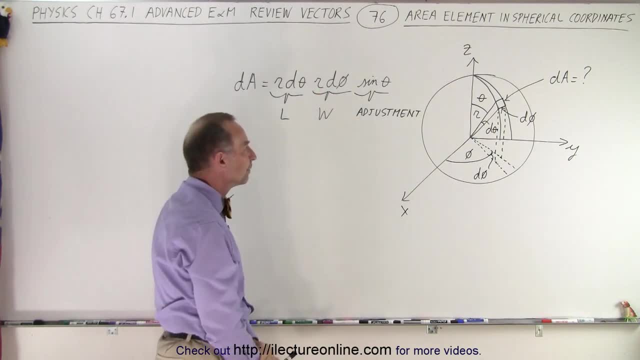 but they don't, because it converges down to a point at the pole. So that is really the area element. We have to take that into account, and that's where the sine of theta comes from. Now, when we rewrite that, we then would write it as: dA is equal to R, times R.